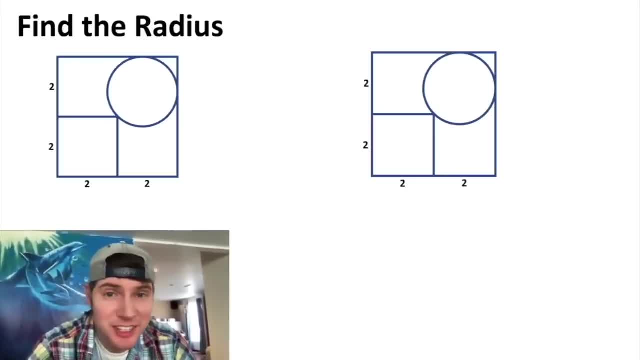 Hey guys, so we want to solve the radius of this circle. First let's find the center of the circle and this right here is going to be the radius. I first thought was maybe it equals one, but it doesn't, because if we bring this down, that's not in the middle here, because the edge of the circle 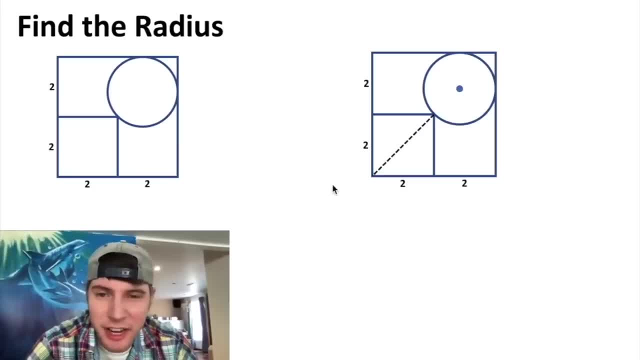 is not in the middle either, So we can't really do that. Next, let's look at this diagonal. here We can actually find out what this diagonal is, because this is a right angle. So if we call this side A, this side B and this side C, we know that A squared plus B squared is equal to C squared. 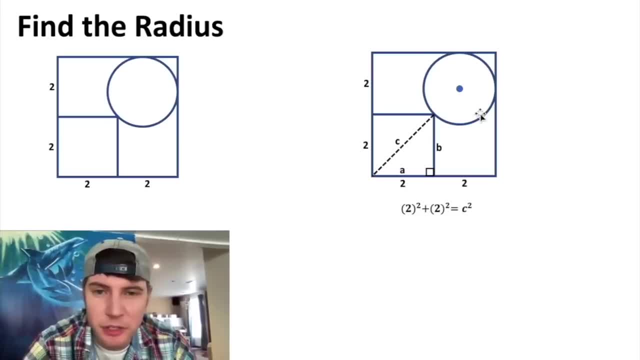 A right here is equal to two and B is the same as this right here, So it's equal to two and C will just leave a. C squared Two squared is four plus two squared is four is equal to C squared Four plus four is eight. We square root both sides. On the left-hand side we can break square root. 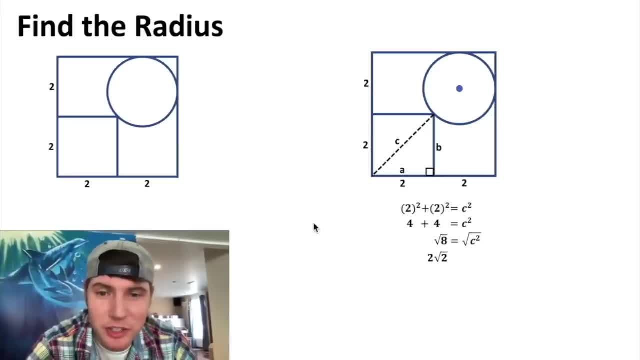 of eight into square root of four times square root of two, and the square root of four is two And on the right-hand side it just becomes C. So we can clean this stuff up up here and let's put two root two right here for this piece of the diagonal. Let's get rid of all this stuff. 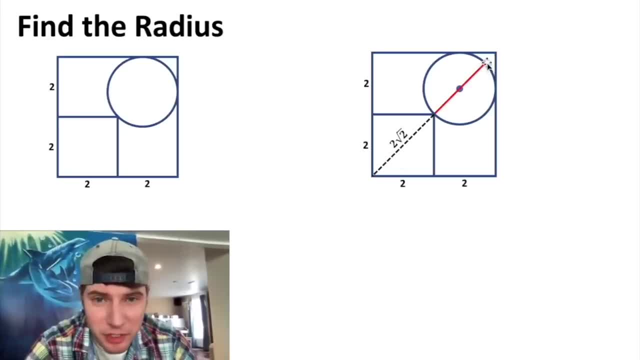 Unfortunately the diameter here is not two root two because it doesn't go all the way to the corner. but we can say that the rest of the diagonal right up here is also two root two, So we can calculate the diagonal. We can calculate the diagonal of the big square and it's going to be equal to the two root two. 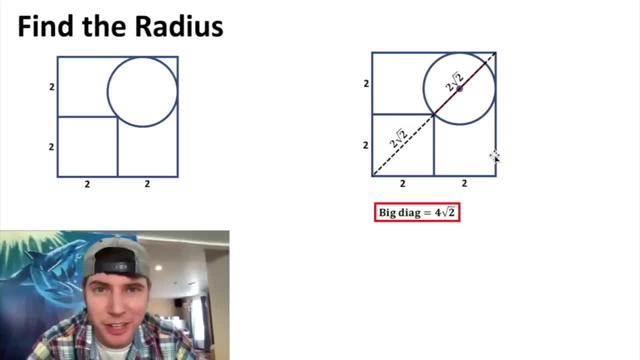 plus the two root two, which is just four root two, And we can put a box around that. Let's clean this all up a little bit. And this right here is the radius. We'll call that R. This is what we're trying to solve for. So we know this, we know this. We just got to find this piece right. 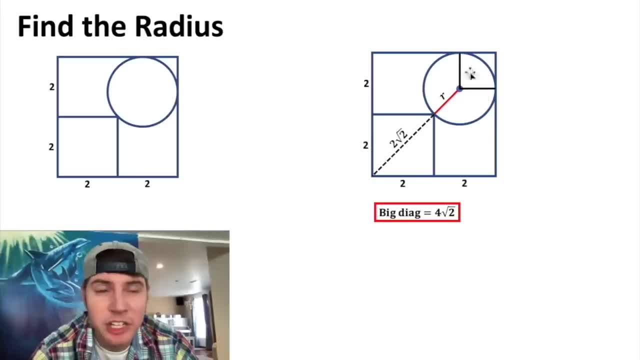 here. Well, that's not too bad, because we can make a square right here. We know each of these are equal to the radius as well, So we can call both the sides of this square R. Then we can do another diagonal. We'll move this R over to here, And if we make the diagonal equal to C, then we know that. 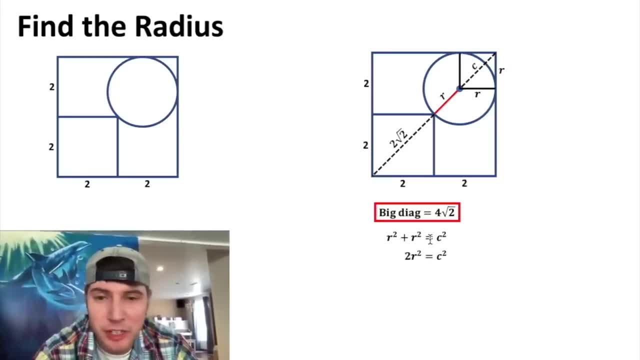 R squared plus R squared equals C squared. Well, R squared plus R squared is two R squared. We can square root both sides. The left-hand side can be broken out into square root of two times square root of R squared And the right-hand side. 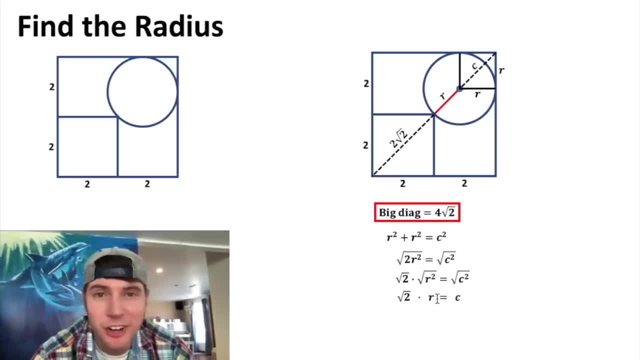 would just be square root of C? squared And the square root of R? squared is just R and square root of C? squared is just C, And we can smush these together and we have: square root of two R is equal to C. Up here was our diagonal C, So we can change that into root two R. Clean things. 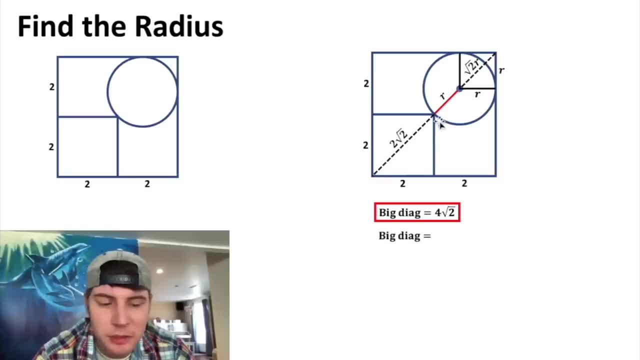 up a little bit. And now what do we have? Big diagonal again. This time it's equal to this diagonal here, the two root two plus the R plus the root two R, And we can put a box around that. We know the big diagonal has to equal the big diagonal, So we're just going to set the four.